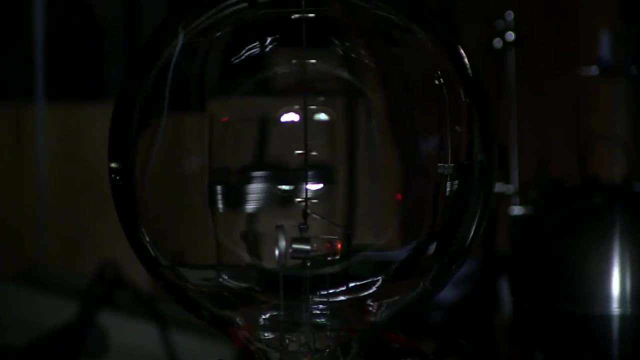 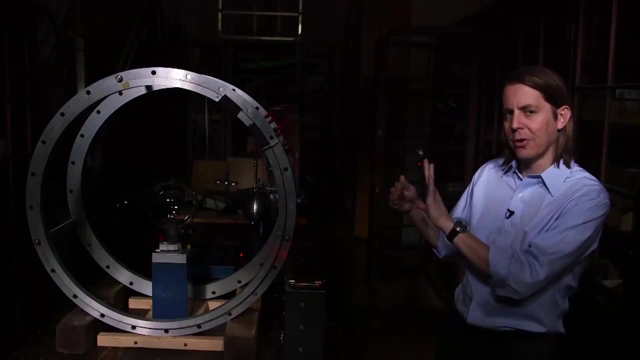 just means a heated metal filament that's easy to draw electrons off of. Near the gun that you can now see glowing orange is a little metal plate that we put at a large positive potential So that sucks the electrons up to a few hundred volts at the plate. The plate has a hole. 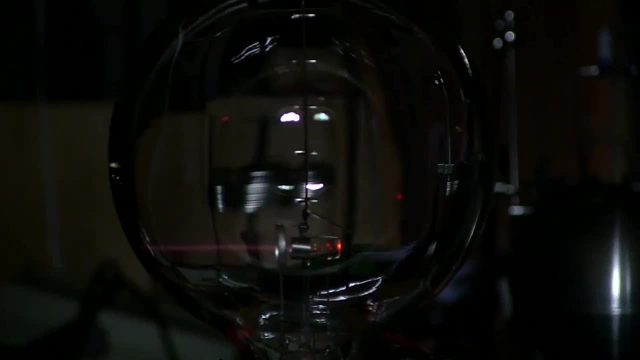 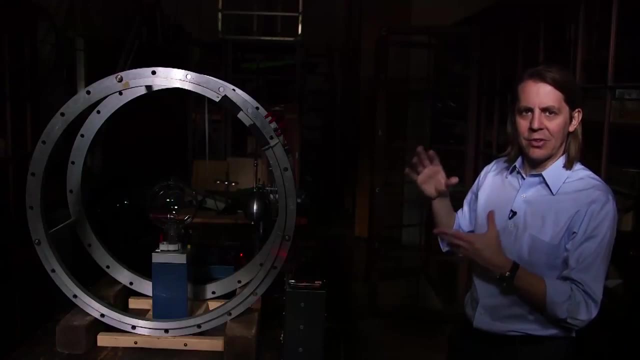 in it so that some of the electrons keep going in form of beam. that continues on until it hits the glass. Now you're seeing the beam because it's exciting a little bit of gas that's inside the bulb, So you're seeing light from the gas, but it's there because the beam is shooting through the 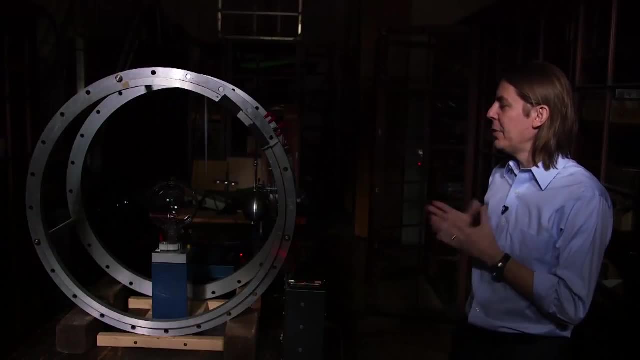 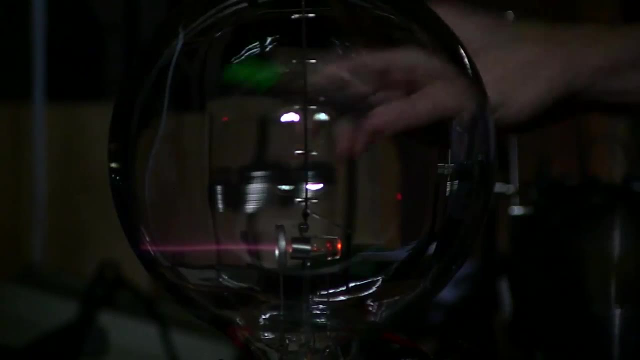 gas. So you're seeing the electron beam indirectly. Now we know that if we bring a magnet nearby it'll deflect the beam. So here's my north-south bar magnet and, sure enough, one pole pushes it up, another pole shoots it down. If I bring it in and do these kinds of things you can. get a little bit more effected. So I just want to show you a little bit here. So this is my north-south bar magnet and sure enough, one pole pushes it up, another pole shoots it down. If I bring it in and do these kinds of things, you can. 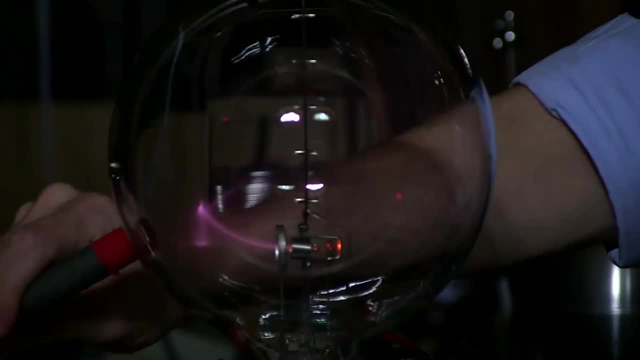 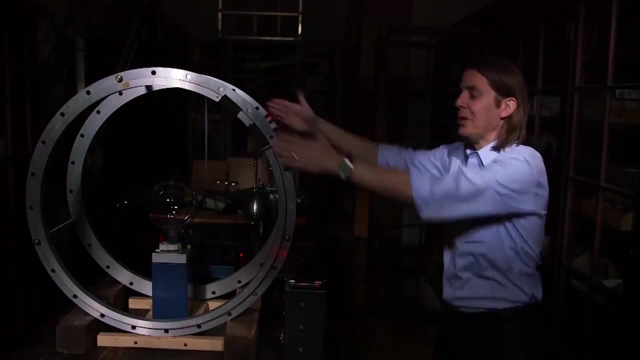 You can do all kinds of crazy patterns with the beam if you bring in a strong, concentrated magnetic field, But what we're here to do is to create a uniform field, and that's what these two big coils are. So this is a large coil of wire on one side of the bulb, large coil on the other side. 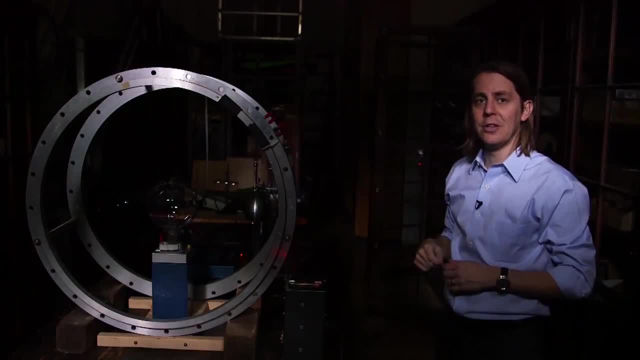 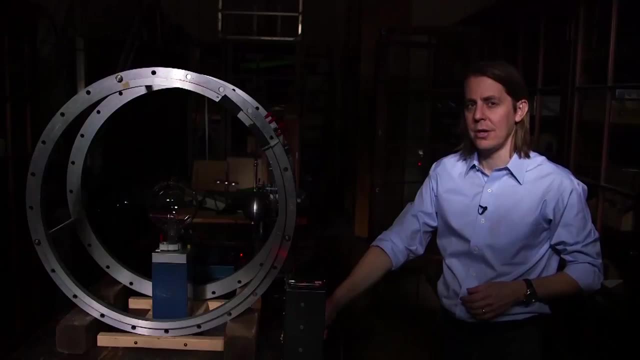 So if you put them together you can make a reasonably uniform magnetic field on the inside. So this power supply is going to increase the current in these coils and we'll see what pattern the electron beam takes. So here we're going to start turning it up and you can see it's starting to curve more. 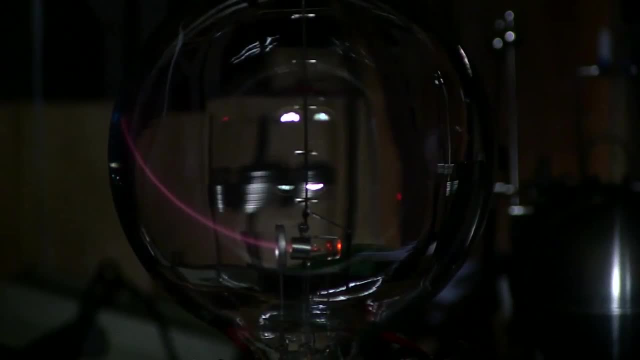 and more, And right now it looks like it wants to make a circle, but the radius is too big, it doesn't fit in the bulb. So if I keep turning it up more and more current, bigger and bigger B field, eventually, there it is. 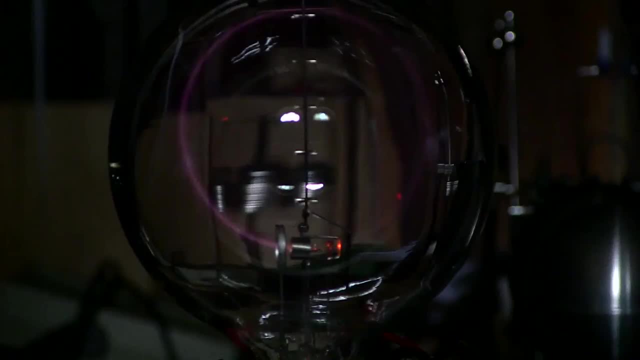 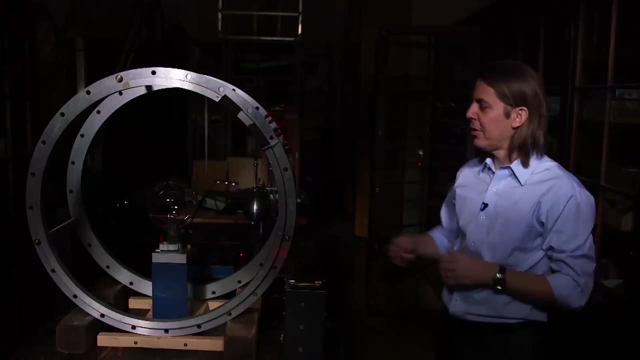 It makes a circle, Perfect circular motion, going right back to where it started. and if I turn the magnetic field back down, back down to zero, straight again. So there's direct visualization of the circular motion of charge in the magnetic field, And that's exactly what we want. So you don't have to be very creative with it. You want to stay safe When you're playing with your vario. You want to stay safe. It's just a matter of playing with your vario And you want to be very, very careful. So with a스� instruction, we're going to be really careful about where we want to go. So with aast, You're going to jump in the vehicle to see what direction you should be moving out. You're going to try to get a spot. but if you're trying to get the right direction, you're going to need to get a spot. I would say you need a bit of time to get a good feel for your vehicle. You're going to want to move a little bit and it's going to be pretty easy right now.